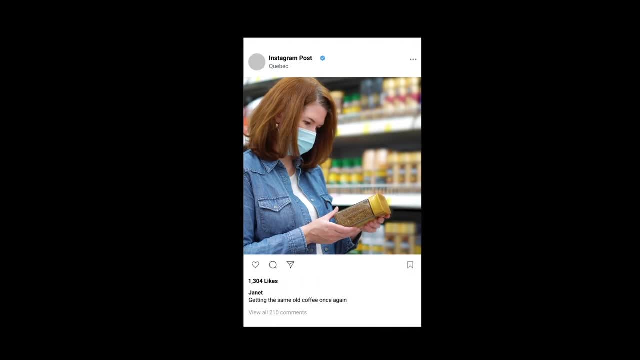 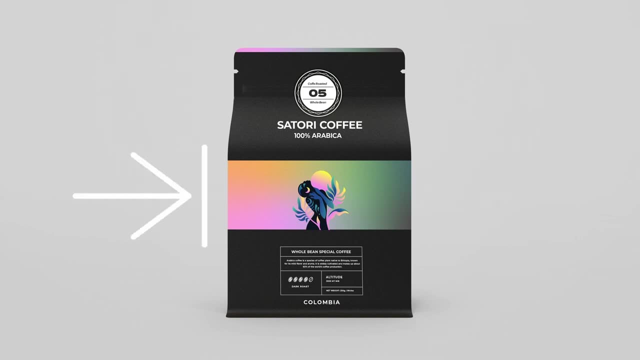 will make the package design differentiate itself from the other generic styles of packaging. now, i did play around with a lot of different layouts and actually i had a band of color gradients which i soon dropped. but at this stage it looks something like this: when people drink coffee, they have that burst of energy and they feel really alive. 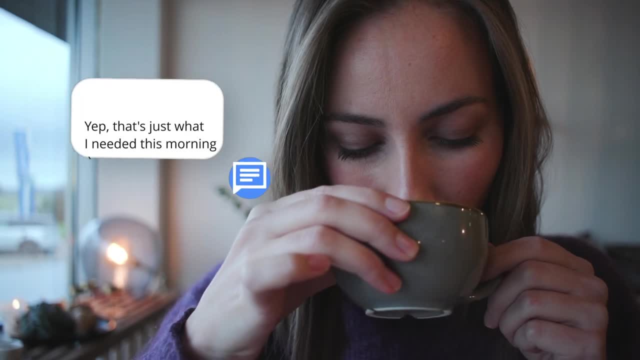 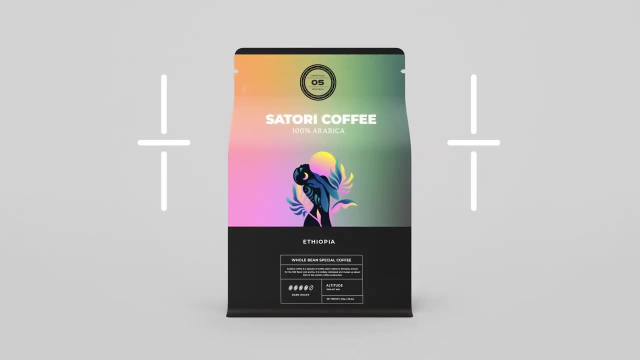 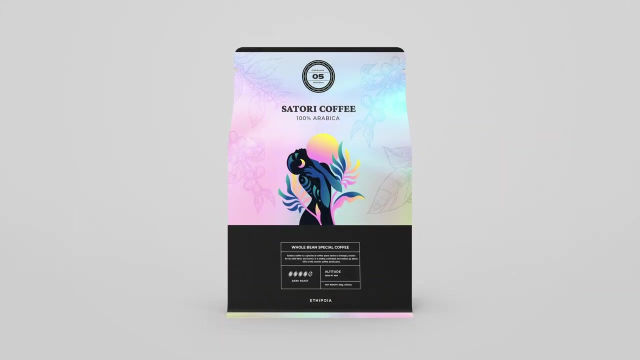 i also think my package design is going to help get that point across. so from there i extended the gradient band over much of my design and i did feel this was heading in the right direction. i then decided to really target that younger generation and elected for a more trendy iridescent color scheme gradient, as you can see here now. i think this does. 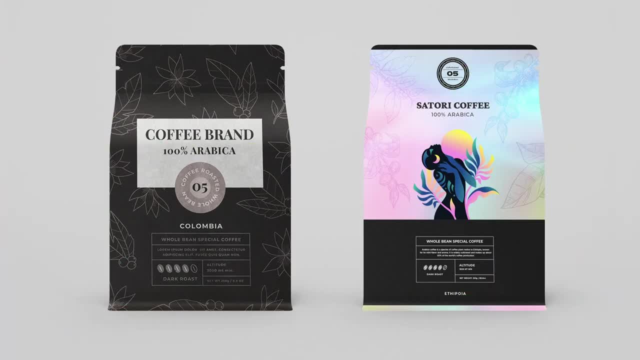 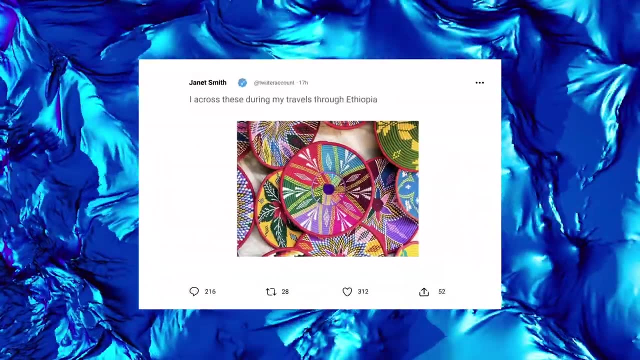 effectively differentiate itself from products that are generic in this category. it points to a vibrancy of the ethiopian culture and how coffee can make us feel when we drink it, and also, of course, it is quite feminine due to the purple hues and so on. i also like how i have a thin 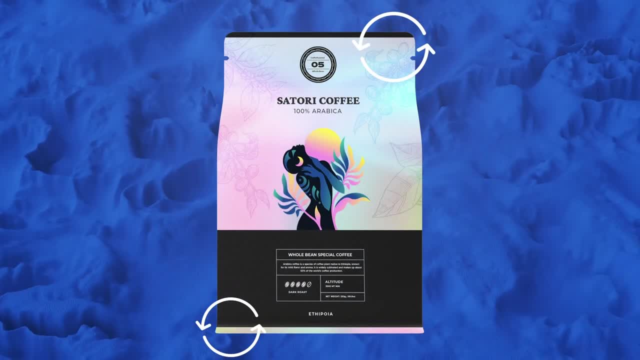 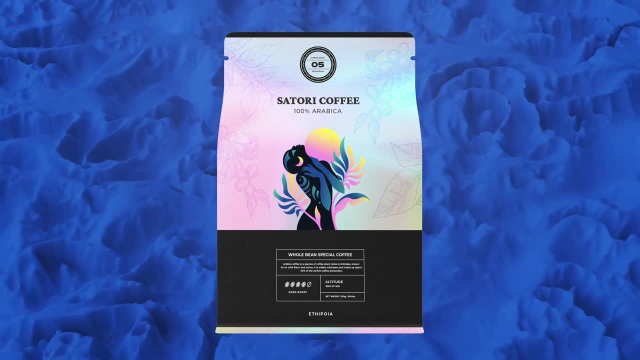 black section on the very top and a thin gradient section on the very bottom. for me, that was a nice touch and a smart move, along with the drawings of coffee beans growing on the sides. so, yeah, this design, for me at least, pulses with energy and vibrancy, which is exactly what i was going for. 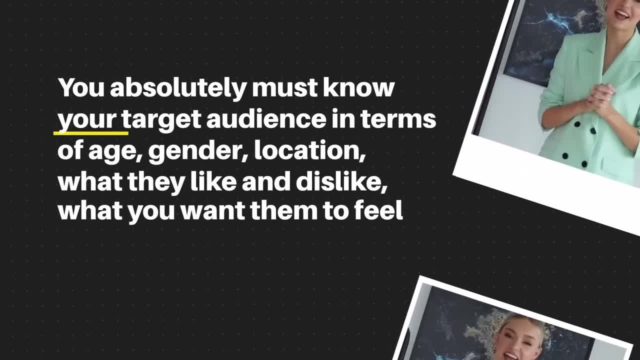 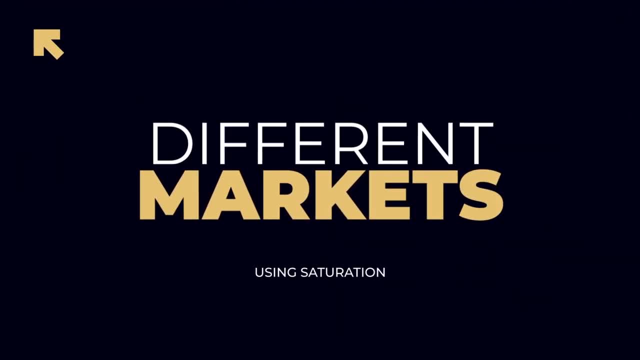 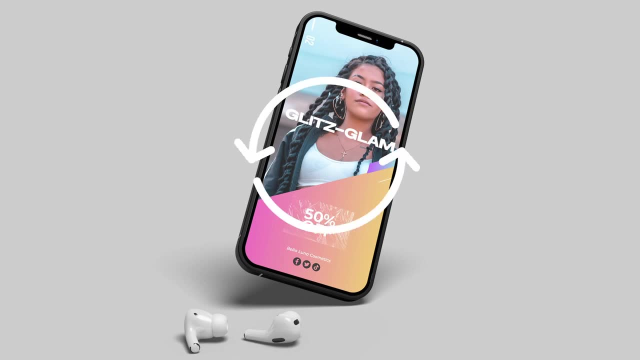 so color can really help to differentiate a product or a design from other ones. but next i want to use color that's going to appeal to two very different markets with saturation. both designs are going to be geared towards cosmetics and we're going to be using social media here. think of it like an 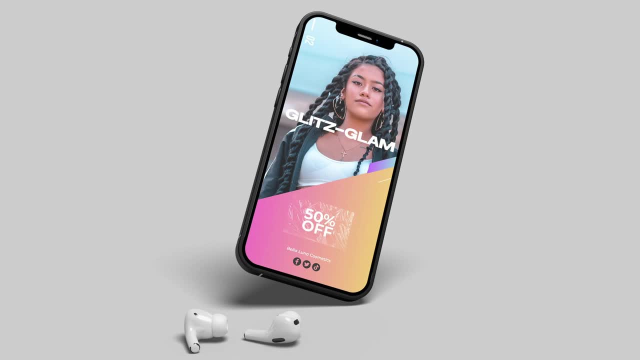 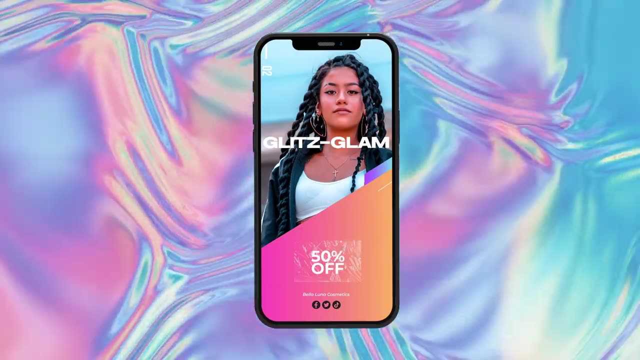 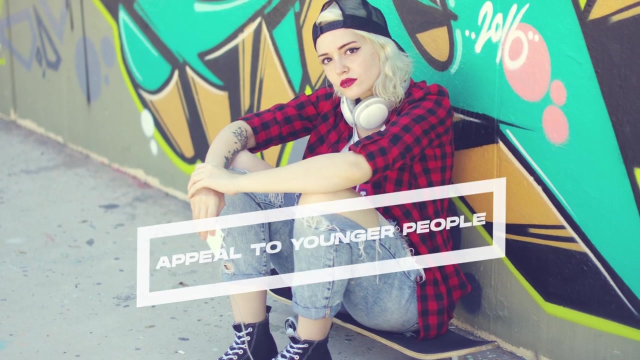 instagram story or whatever. so the first design uses bold and bright colors, and this can sometimes seem tacky or cheap. however, in this instance, they would make a cosmetics product potentially appeal to younger women, perhaps even teenagers, and that's due to the high saturation of color, and that makes 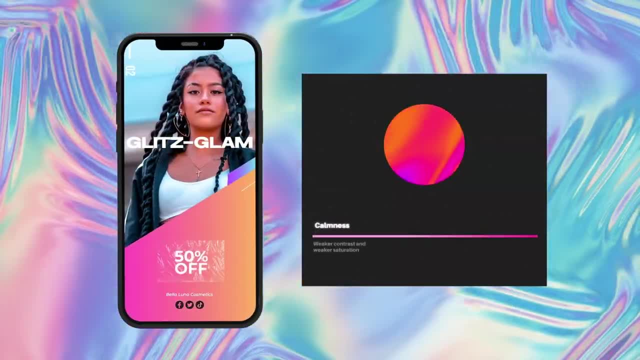 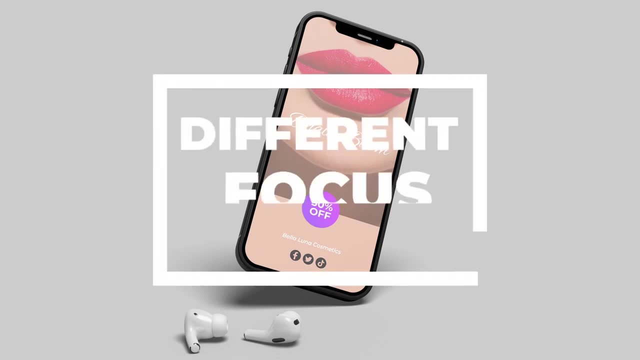 the design look more fun, more striking, more bold. but if we go ahead and flip things around completely to a more muted color palette in terms of saturation, now the entire design has a different focus. now things are more calm, more refined, more elegant, and this design would appeal to women. 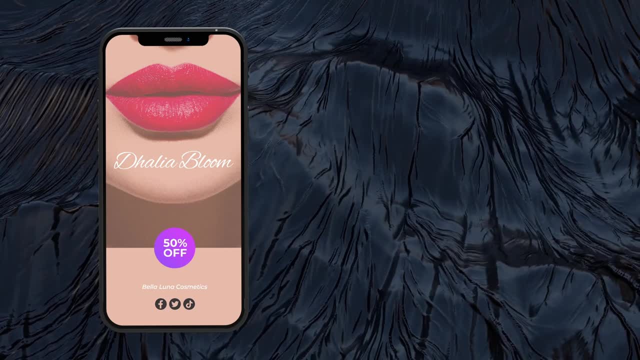 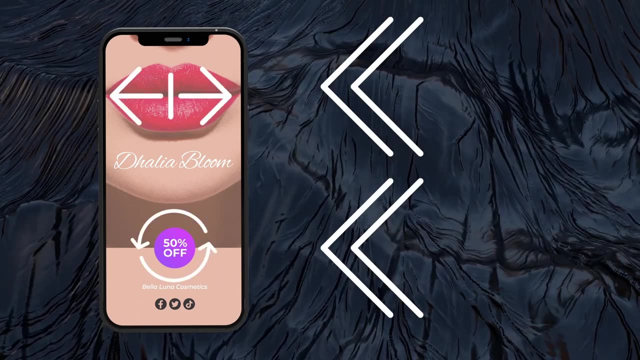 above and beyond their 30s and potentially to sophisticated middle upper class people. but we do have some areas of high saturation, including the cta, and of course, the lips, and the lips are the product. so we do obviously want this to stand out a little bit more. 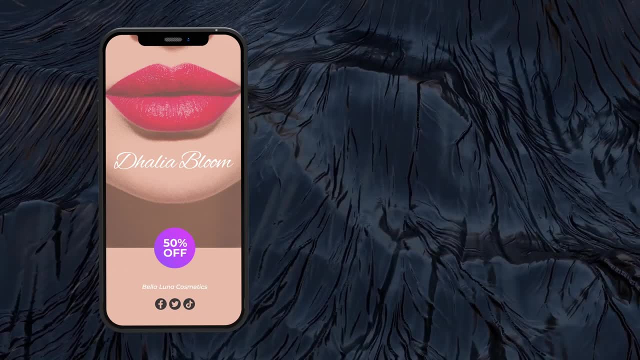 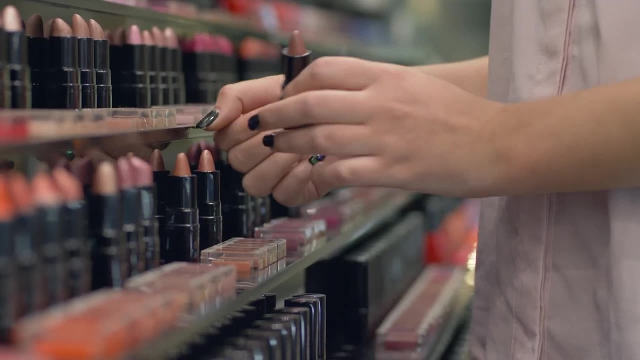 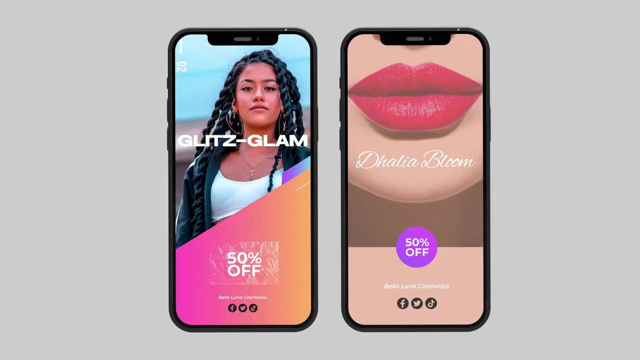 but in general, lowering saturation and contrast will give a more refined and more calming look to your design, and this is often perpetuated by cosmetic brands throughout the entire industry. but again, it does depend on your target audience, the demographic, and that's demonstrated right here. so here's a banner for a hotel notice: the typography: 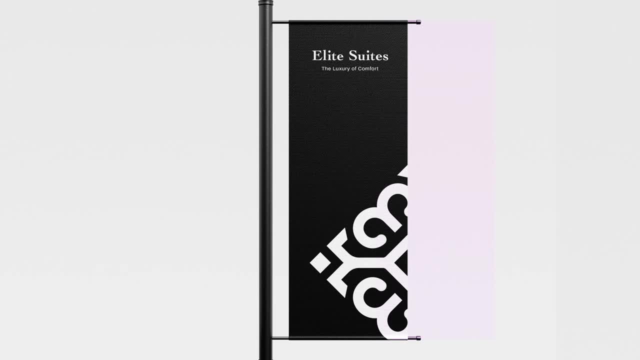 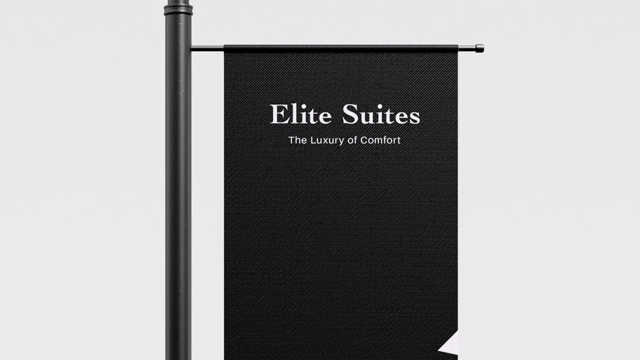 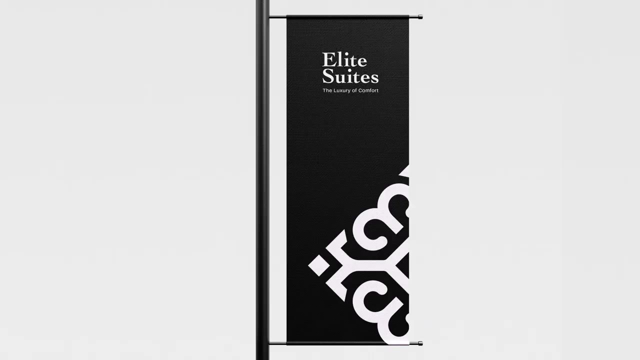 reads elite suites. that would suggest a higher end kind of hotel, and the fact that we have a serif font and a clean, minimal layout just pushes that idea even more so. with that in mind, what color scheme can we run with on this design? the truth is that many color schemes would. 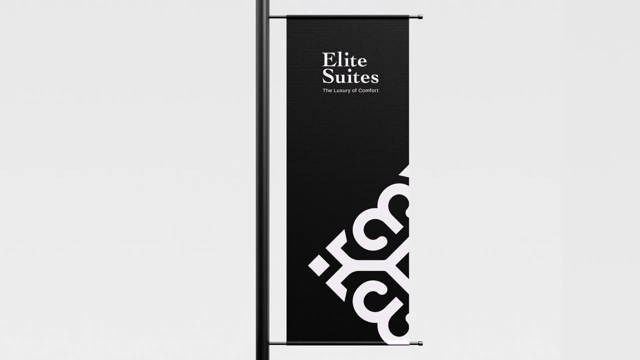 actually work and it would depend on the market research this brand actually conducts. but at the same rate, there are many kind of schemes that wouldn't work and would just fail. one scheme that would work, in my opinion, is gold and purple, and we all know that gold suggests luxury. but matched up. 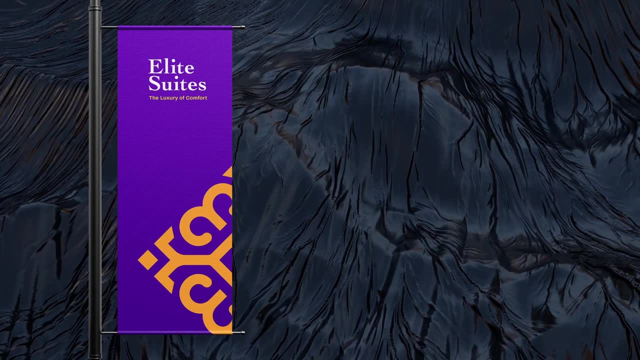 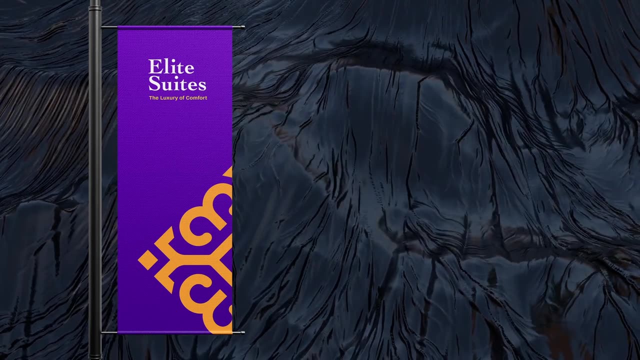 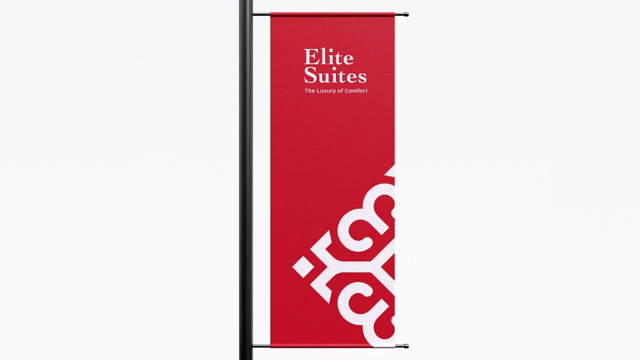 we get a kind of royal or regal feel. the purple is calming and this works well for a business such as hotel suites. we all want peace and calmness when we check into a hotel- well, most of us anyway. now, i think another potential color scheme that could work here would be red and white. the reason 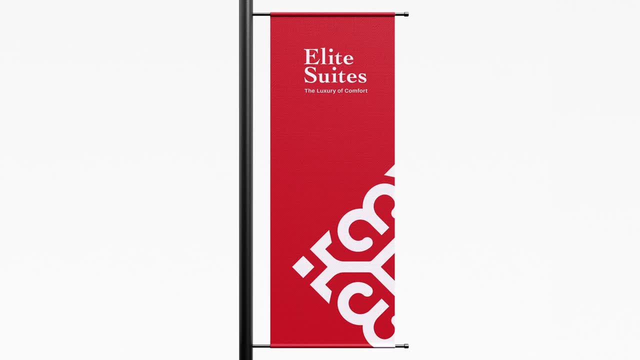 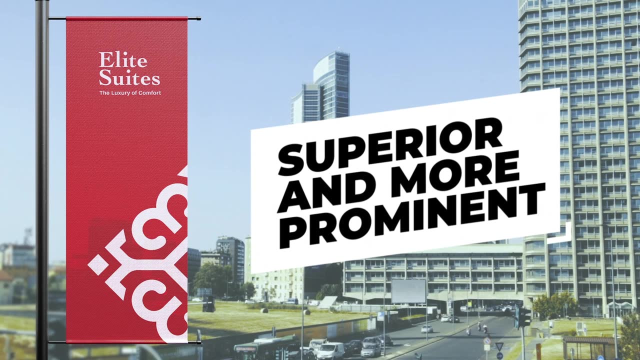 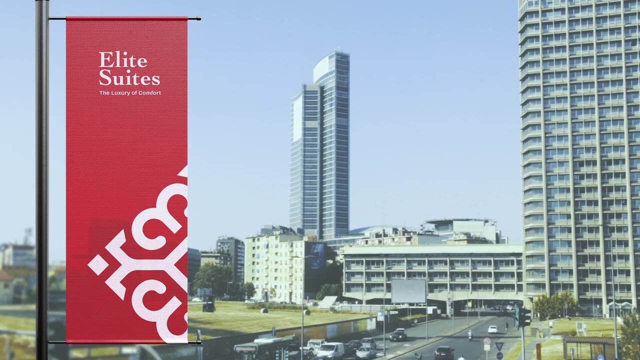 being is that red is very attention seeking and imposing. this hotel might actually consider itself to be superior and more prominent, and so a bold choice like this in color could actually work really well. again, it depends on the research and what direction the branding team would actually want to take it and who they're targeting. but, as you can see, color can totally change your design. 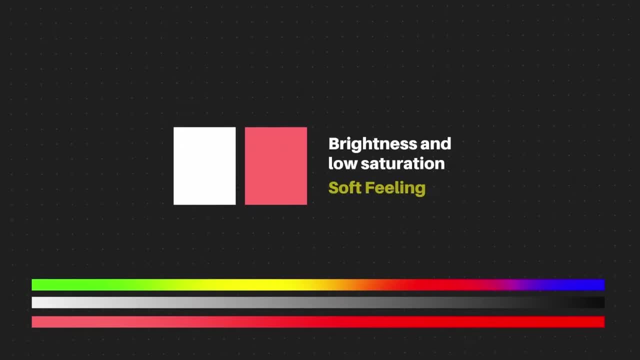 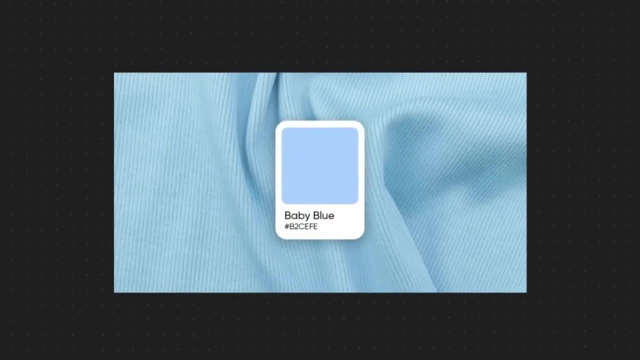 and that's why it's so important to know who you're targeting and why. then you can actually allow the color to do the talking for your design. now you can learn a lot more about color in graphic design simply by clicking that video on the screen. but until next time, guys design the future today. peace you.